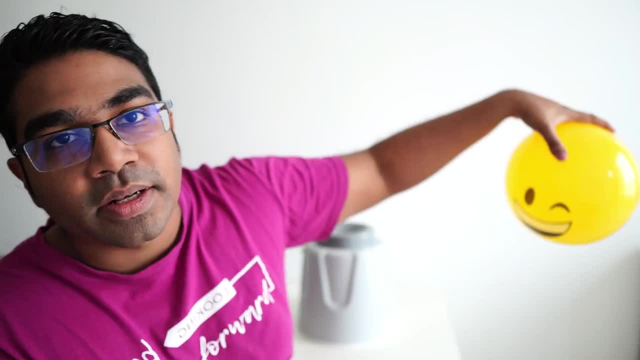 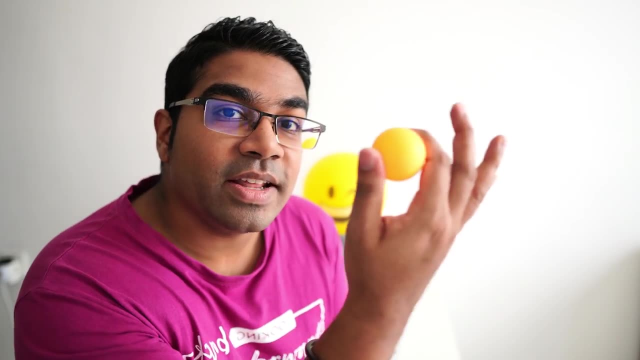 then the electron will instantaneously leave the metal. The moment the photon hits the electron, it will leave the surface of the metal. And now we need to discuss the energy of the photon. The energy of a photon is directly proportional to its frequency and the equation relating 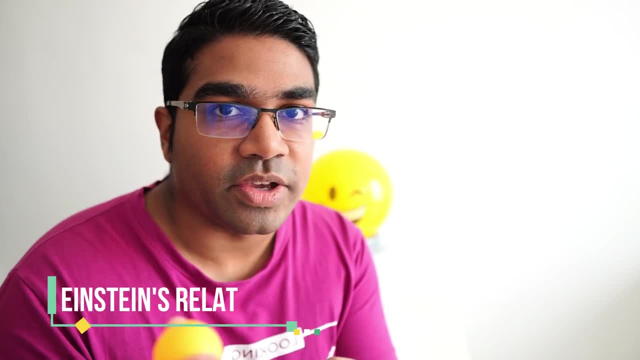 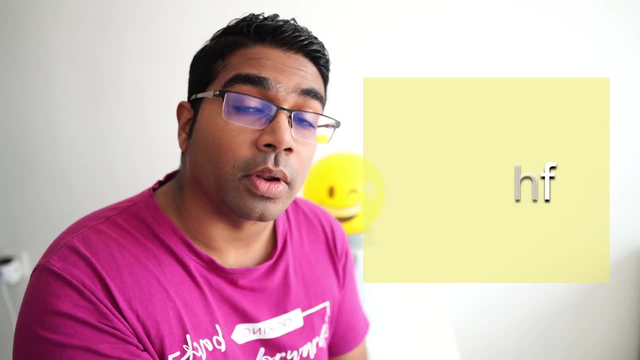 the energy of the photon to the surface of the metal is equal to the energy of the photon. The energy to the frequency is known as Einstein's relation. Einstein's relation states that E, the energy of the photon, equals to HF, the frequency of photon, where H is known as: 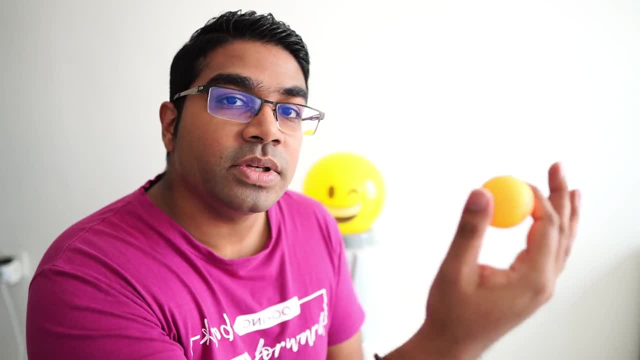 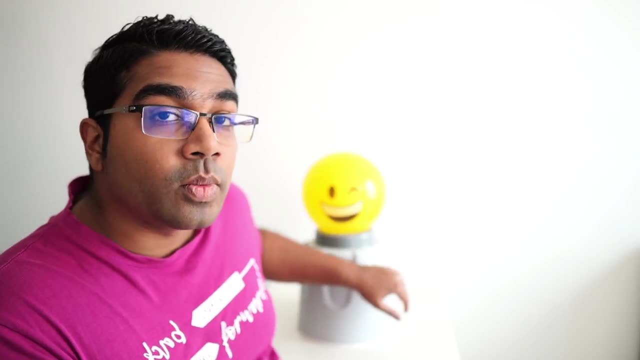 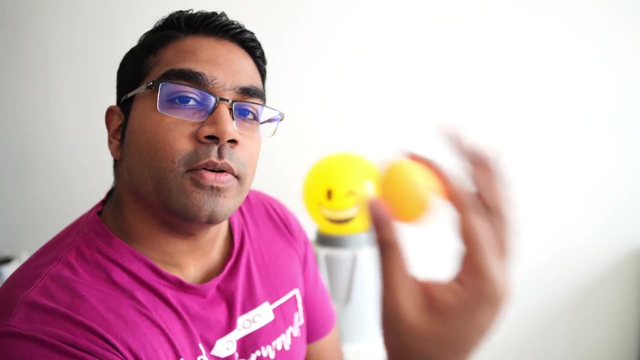 Planck's constant. So we know that the higher the frequency of the photon, the higher the energy contained by the photon. Each metal has a different amount of energy that is required to remove the electron from its surface. Let's say this is metal X and we try to use a photon. 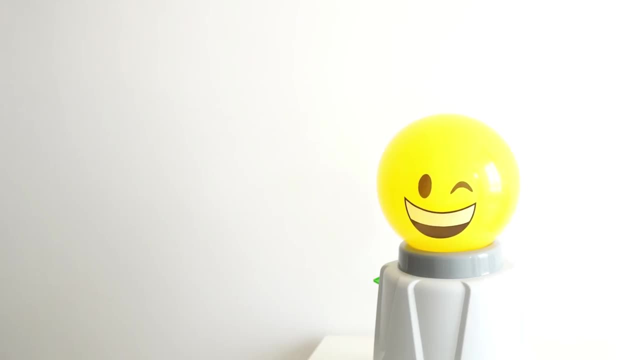 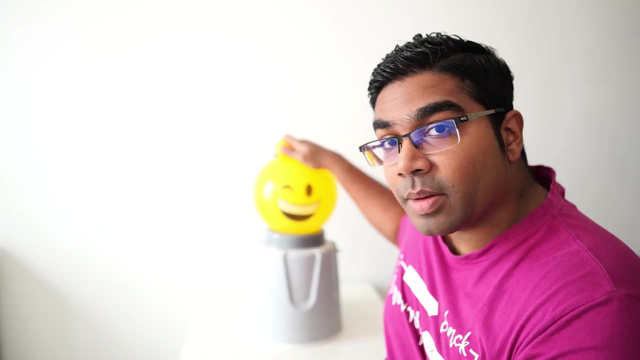 to remove the electron from the surface. You can clearly see that the photon does not have enough energy to free the electron from the metal surface. Once the photon knocks the electron, what happens is that the photon is completely absorbed by the electron and the photon ceases to exist. 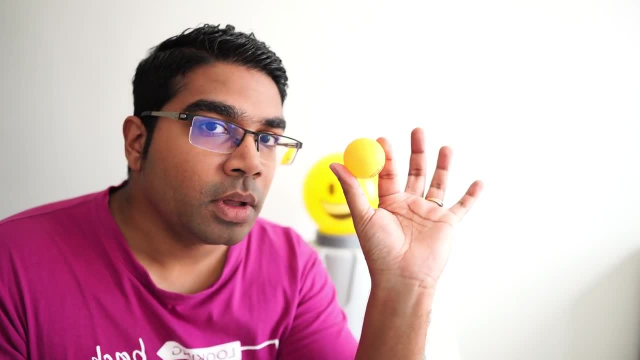 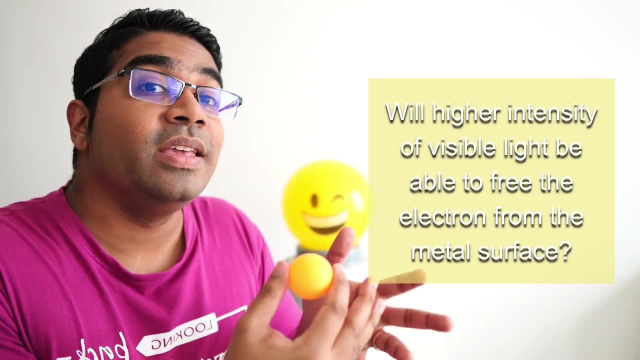 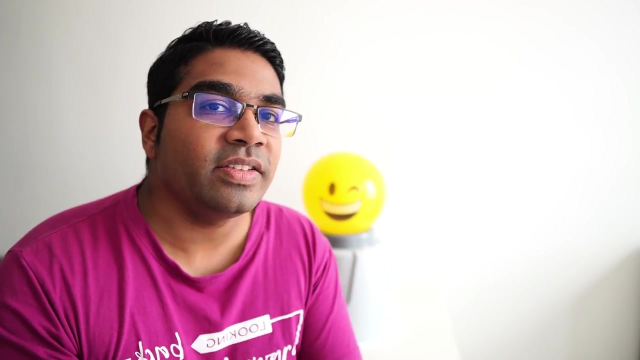 So what happens if we try to use the same photon but with higher intensity? For example, if this was a visible light photon? what if we increase the light intensity? When you increase the intensity of the electromagnetic radiation, what happens is that you are only increasing the rate at which the photon collides with the electron. 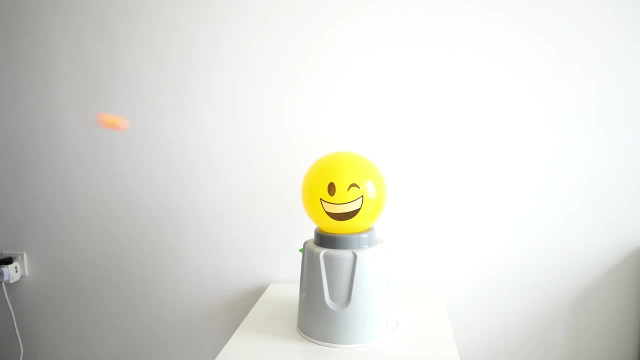 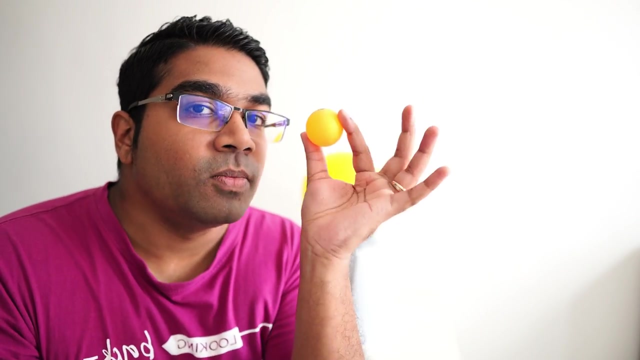 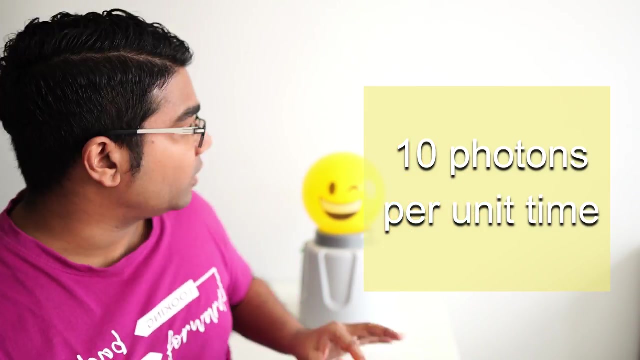 This is still a one-to-one interaction. No matter what the intensity of light at one point of time, only one photon will be able to collide with one electron. Let's say, a low intensity of light results in 10 photons colliding with the electron. 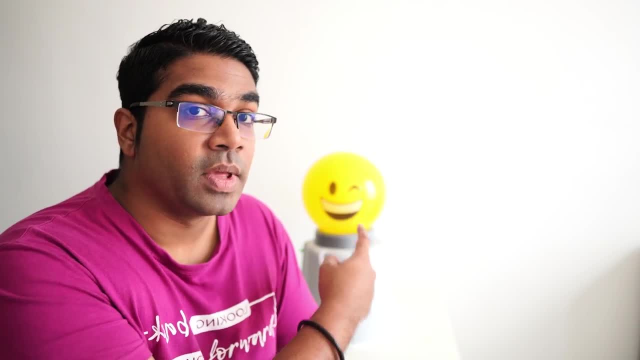 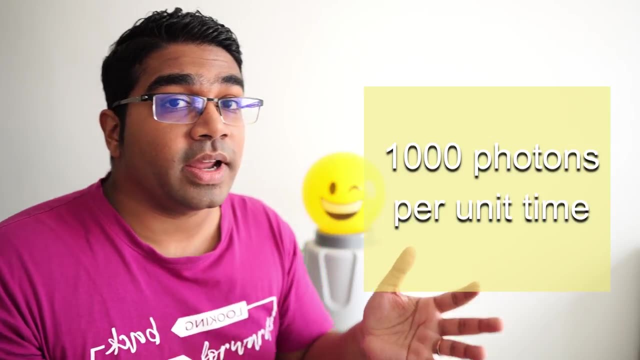 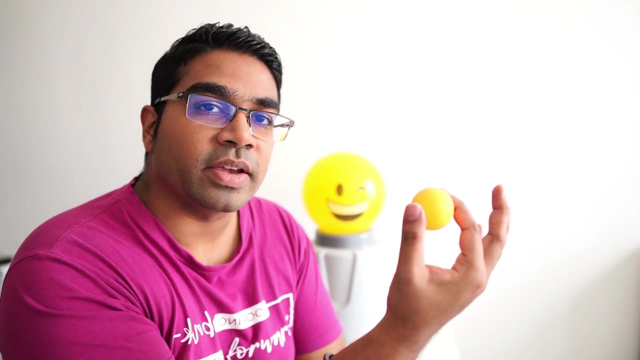 Each photon will be colliding with this electron separately. It is a one-to-one interaction. Let's say we increase the intensity of light and a thousand photons arrive and collide with the electron in one unit time. Still the interaction is the same. It is a one-to-one interaction. 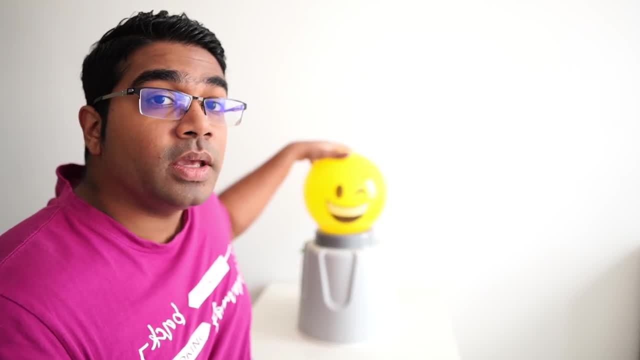 No matter how many photons collide this electron in one unit of time, the photon simply does not contain enough energy to remove the electron from the surface. This is still a one-to-one interaction. No matter how many photons collide this electron in one unit time, the photon simply does not contain enough energy to 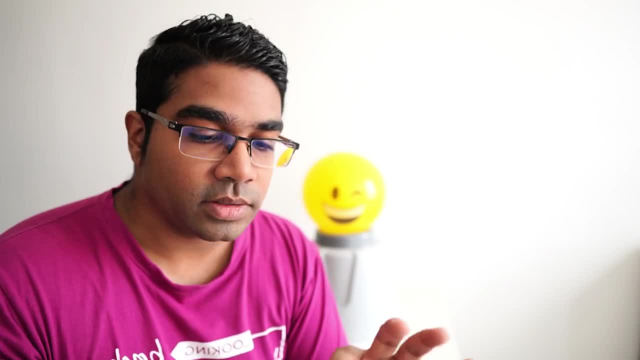 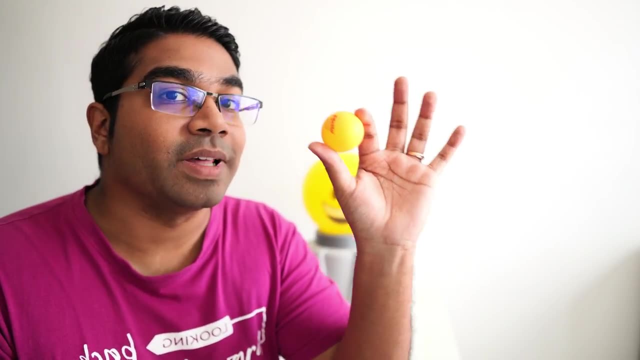 knock the electron off the surface of the metal and therefore the answer is to use a photon with more energy. From Einstein's relation we know that in order to get a photon with higher energy, we need to use a photon with higher frequency. So let's choose an ultraviolet photon. Let's say this: 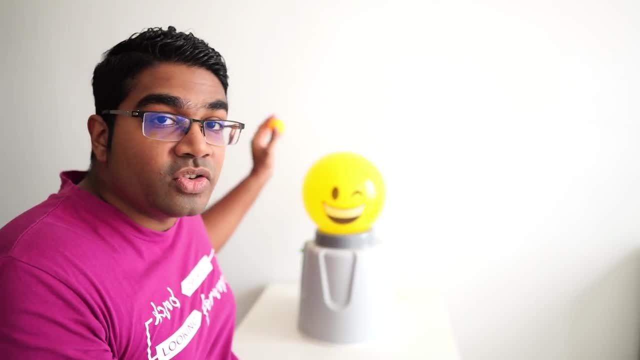 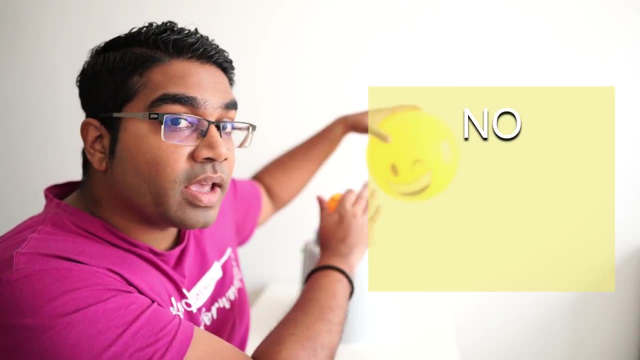 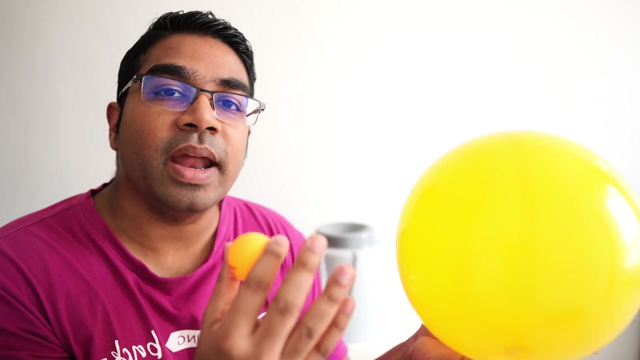 ultraviolet photon has just enough energy to knock the electron off the metal surface. So now we have the electron free from the metal surface, but this electron has no kinetic energy Because the photon only has enough energy to knock it off the surface. This minimum energy required. 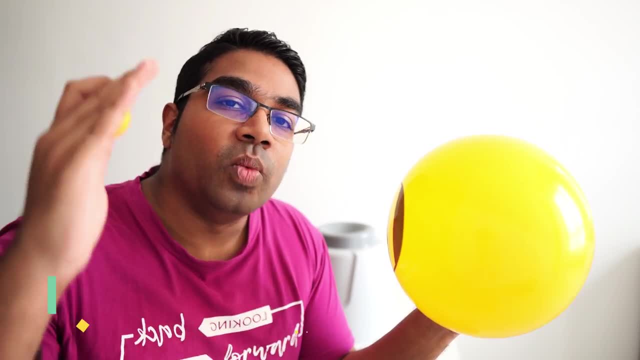 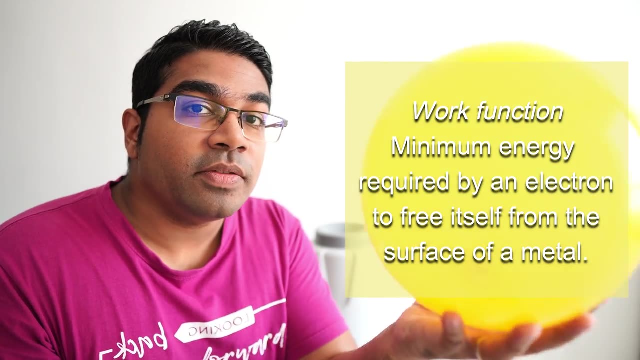 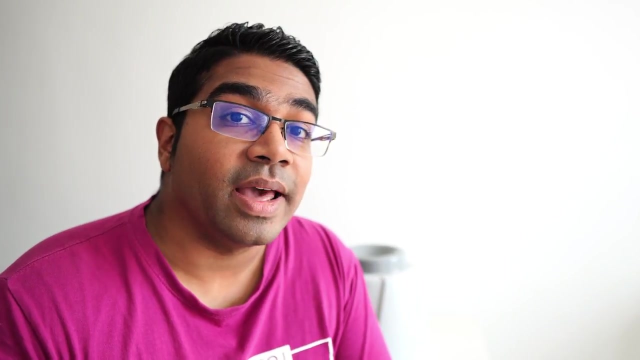 to knock the electron off its surface is known as the work function. The work function is defined as the minimum energy required by an electron to free itself from the surface of the metal. Since the energy of a photon is directly proportional to its frequency, this means that there is also a minimum frequency of photon that will result in the photoelectric effect. 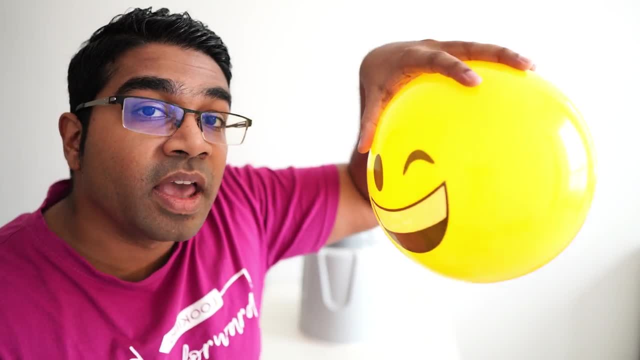 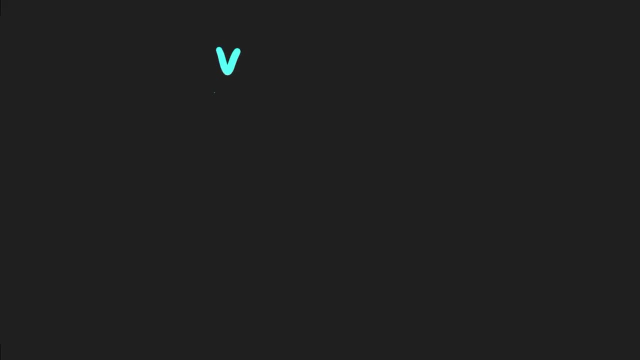 That will result in this electron being freed from its surface, and this minimum frequency of photon is known as the threshold frequency. From the wave equation v is equal to f lambda. we also understand that the frequency of an electromagnetic radiation is inversely proportional to its wavelength. 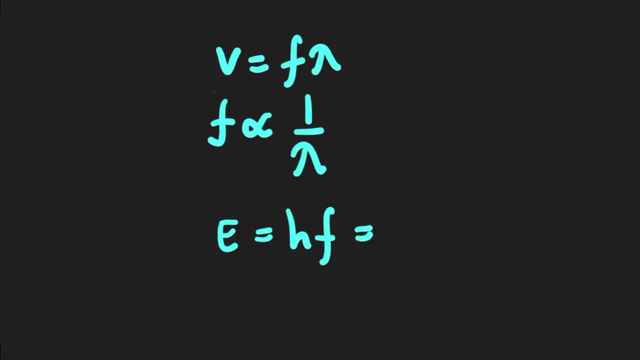 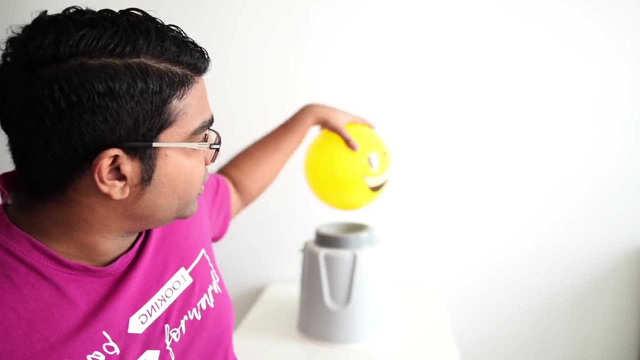 This means that, together with the threshold frequency, the minimum frequency, there is a maximum wavelength to enable the photoelectric effect to occur, To knock the electron off the metal, of the surface of the metal, and this is known as the threshold wavelength. Let's 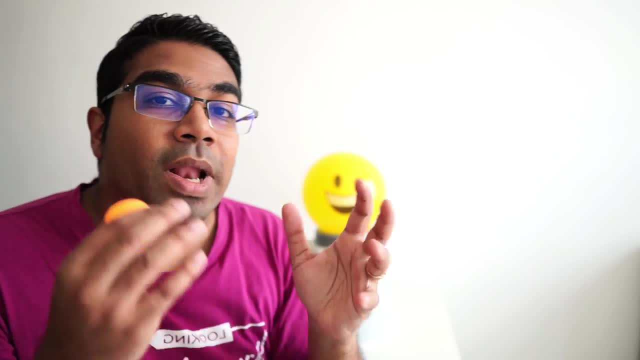 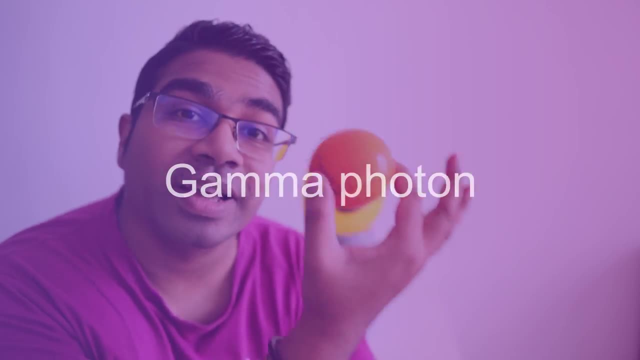 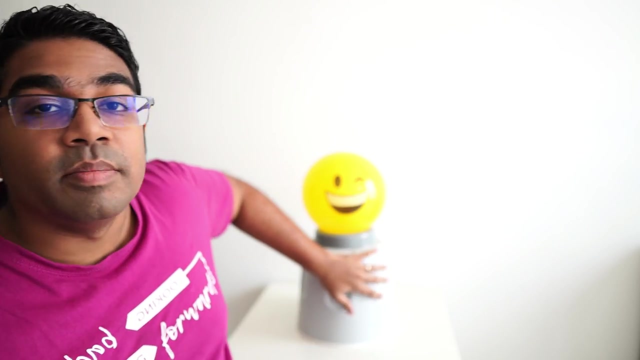 put the electron back on the surface of the metal. What will happen if we use a photon with even more energy than the UV photon? Let's use a gamma photon. This gamma photon has energy more than the work function of this metal Work function. 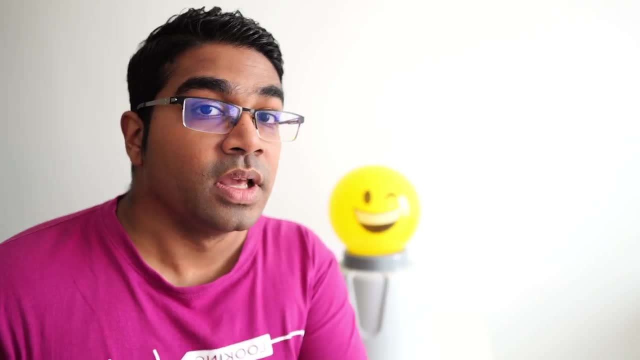 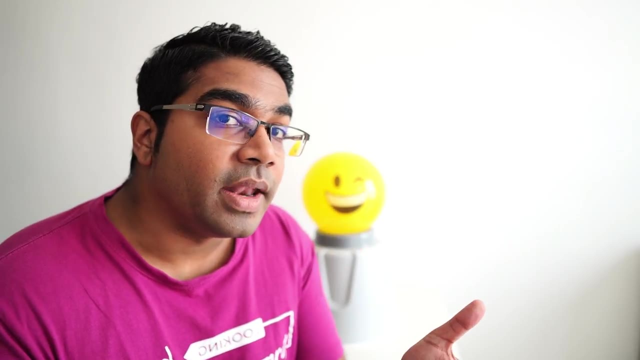 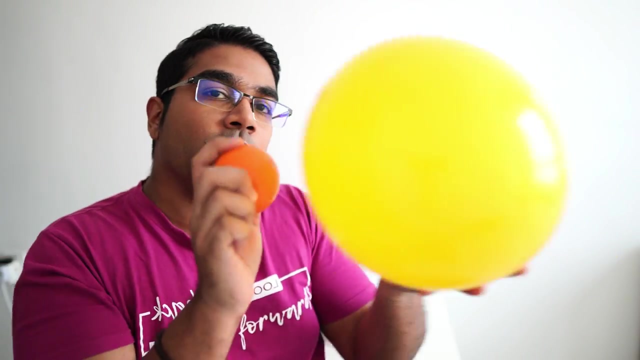 is a property of the metal. Each metal has its own work function. So let's say the gamma photon has more energy than the work function of this metal X. What happens then? You can see that the photon not only managed to knock off the